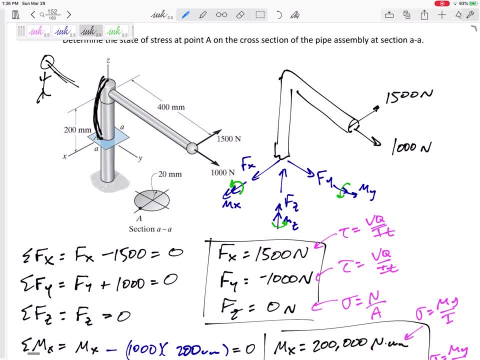 It would bend towards me if I'm looking at it from behind there. All right, it would bend towards me if I'm looking at it from behind. Think about compression and tension. There would be some compression on this side of the beam. There would be some tension on this. 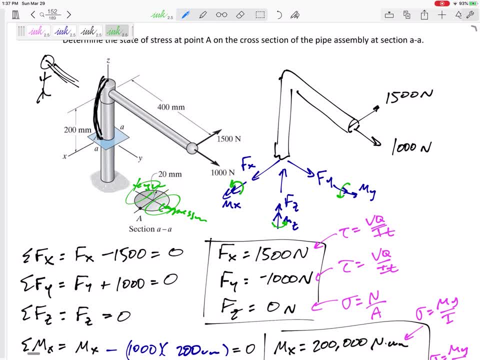 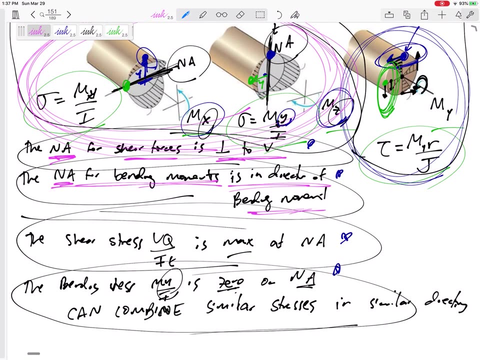 But at point a there would be nothing. There would be nothing. I should have drawn. this is my neutral axis, right there, The x axis is my neutral axis. Let's kind of go back to these neutral axes, The neutral axis where the bending moment is the bending moment. 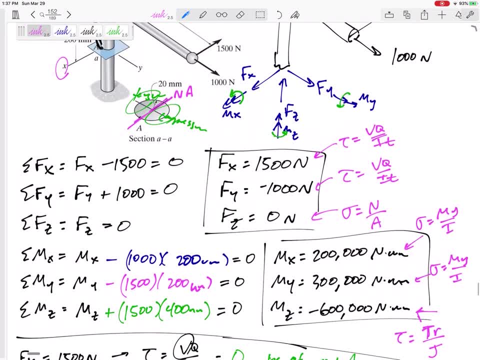 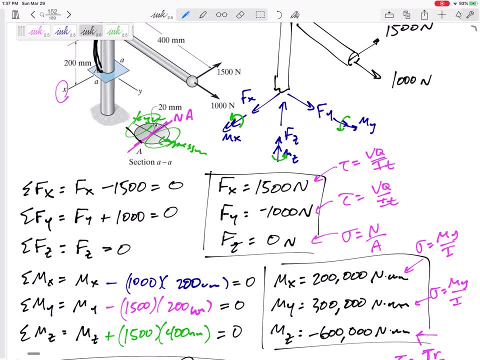 is the direction of the bending moment. So for my x bending moment, x is the neutral axis. One side of it is gonna be compression, one side of it is gonna be tension. but the value at the neutral axis is zero, Herezero, zero, zero, zero. 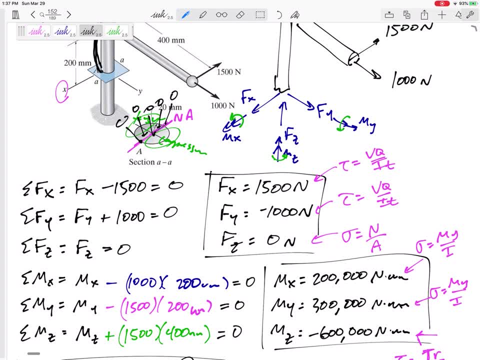 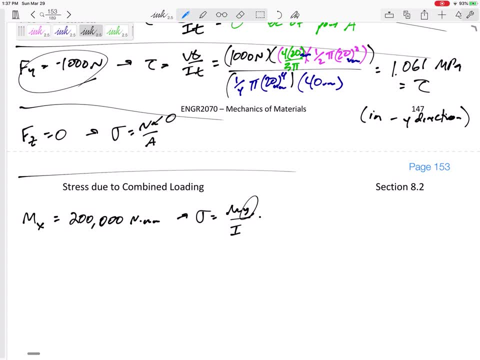 Anywhere on the neutral axis is gonna be zero. You can think about that, because the y, that's the distance from the neutral axis to the point you're interested in. well, that's, if it's on the there, it's gonna be zero. 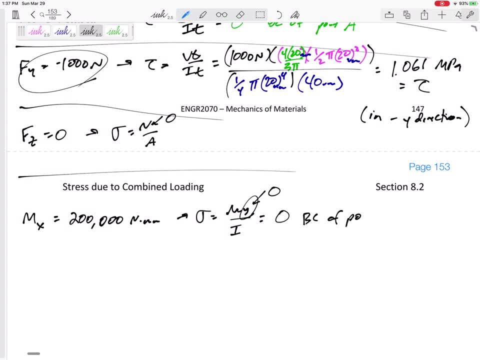 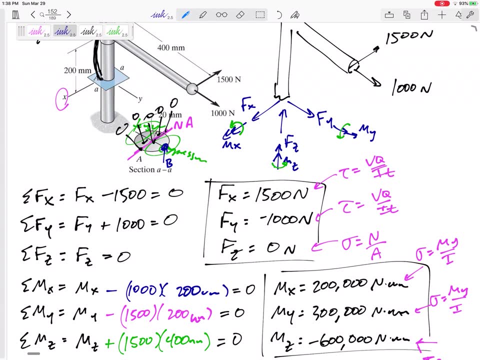 zero. So this is zero because of point A. You know, if it was at point B, right here, it'd be compression And I'd do the MY over I. If it was at point C, over here, it would be tension And I'd. 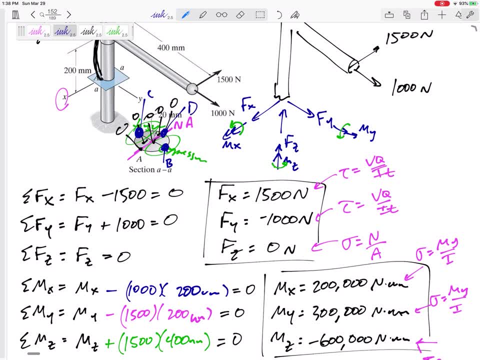 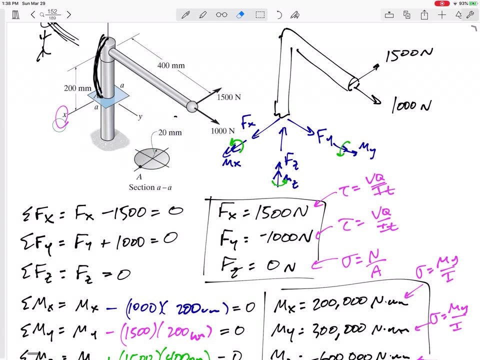 do the MY over I. If it was at point D over here, it would still be zero, just like it is at A. All right, So this moment, even though there is a moment there at point A, there's no stress due to it. Okay At point or sorry. let's look at the next moment, the moment in Y, The moment in: 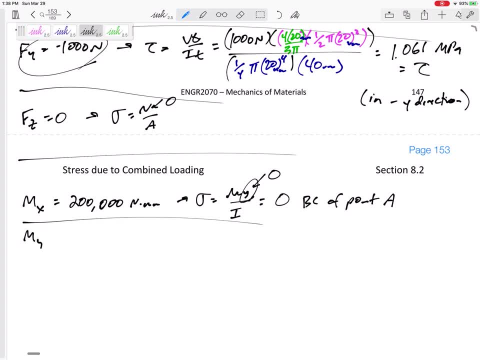 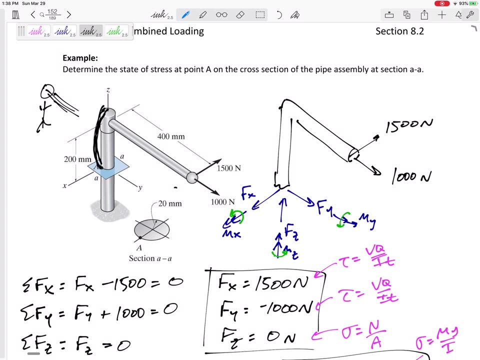 Y MY is positive 300,000 Newton millimeters. It could create an MY over I, So let's think about a Y bending moment, All right, So this, this that I drew, this bending, it would bend towards this person. 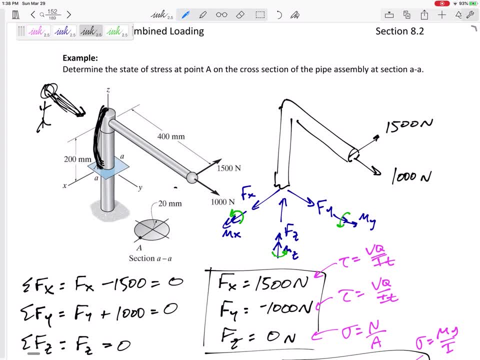 Looking at it from the backside if that's a Y moment, But sorry, that was the next moment, That was the next moment, That was the next moment. But my Y bending moment, my Y bending moment, would cause this to bend, sorry, would cause this to bend this way. 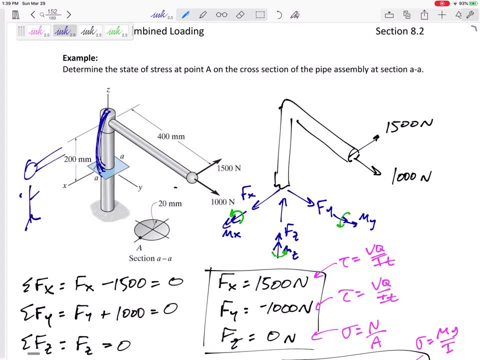 towards a person looking at it from here. Right, It would cause this to bend this way. Put your thumb in the positive Y direction, kind of bend that pool noodle, and it would bend out this way. It would bow out right Over here. it would be tension Over here it. 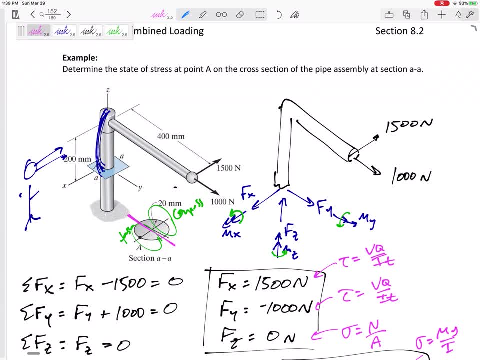 would be compression. Let me draw that neutral axis Right there. the neutral axis for bending moments is the axis, is the Y axis. So for a Y bending Y moment, that Y is the neutral axis. So there would be nothing on the neutral axis. But yes, over here, out at A, there would be an M. 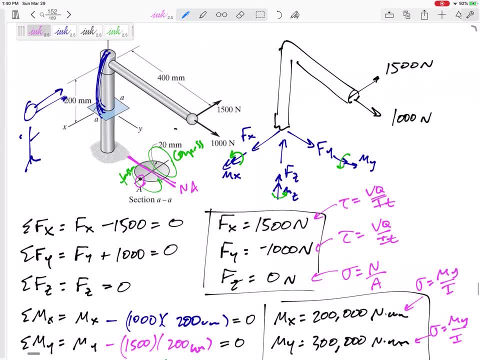 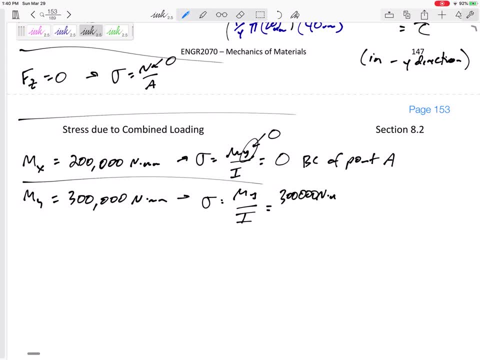 Y over I at point A. If look at point A there will be an M? Y over I. The M-300,000 Newton millimeters, The Y? Y is the distance from the neutral axis to the point I'm interested in That. 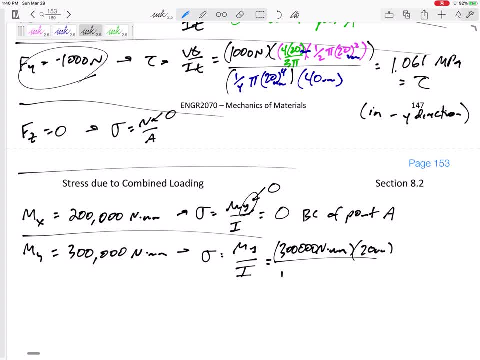 would be 20.. Right, That would be the radius And then the I. I've already calculated that Somewhere one 4th pi R to the 4th Right, And then the I: 0.4 pi R is the distance from the. 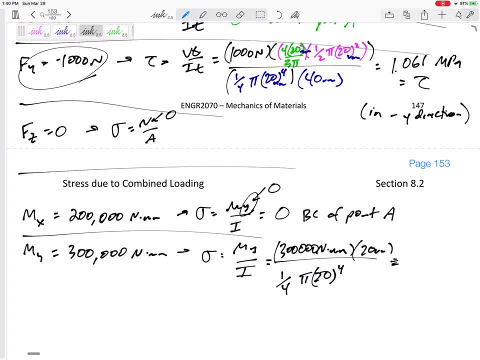 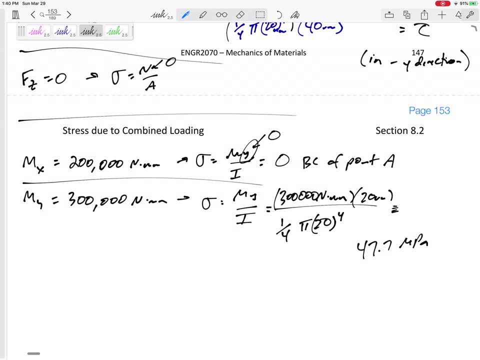 neutral axis to the point I'm interested in, That would be 20.. Right, That would be the radius, And the fourth, uh, this, i would get to be 47.7 mpa. uh, it is a sigma, not a tau, it's a normal stress sigma. 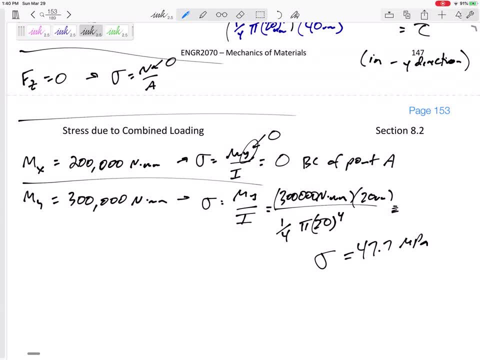 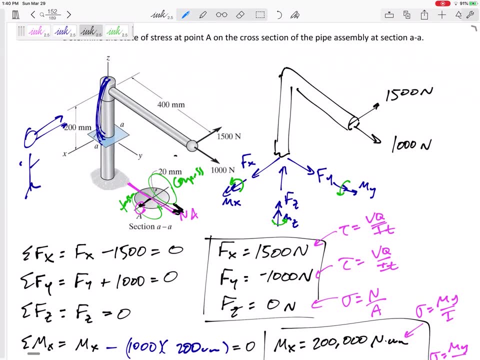 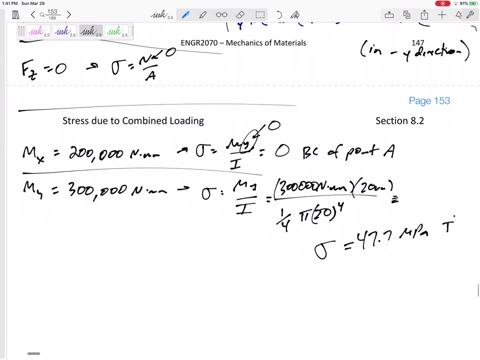 and uh, tension or compression, tension or compression. could you see that a positive y moment would cause compression? i start with compression. positive y moment would, would pinch in this half of it, but it would be tension in the half that i'm looking at for part a. it would be. 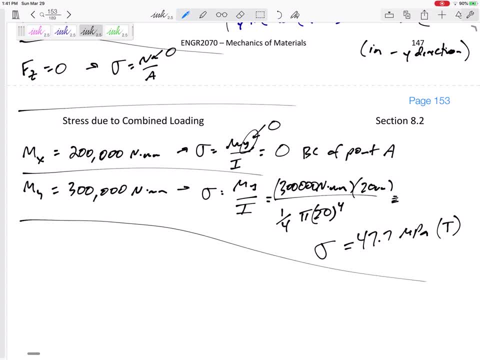 tension. okay, all right. and then, last moment, we're almost there. you can see the light. all right, last moment, mz, mz of negative six hundred thousand newton millimeters. it could cause a shear stress of t over j. uh, what would that look like? uh, a negative z moment. 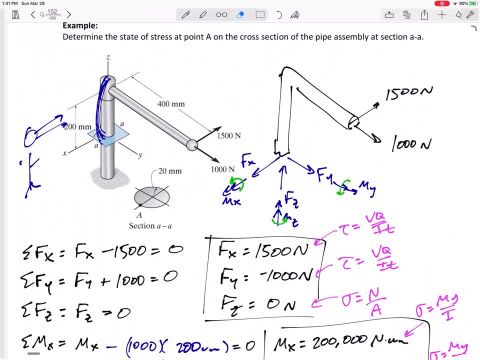 a negative z moment. a negative z moment wouldn't bend it, it would twist this beam. a negative z- think about using my right hand- uh, negative, let's see, that would be positive z, negative z would be that way, that way, that way. that type of shear stress, that type of shear stress. 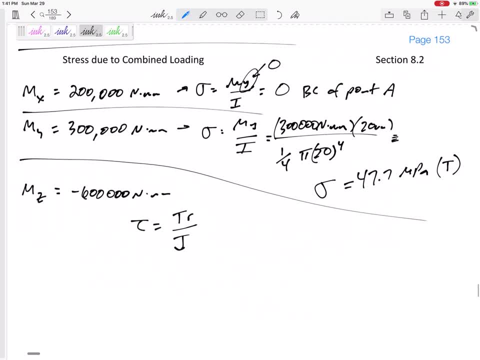 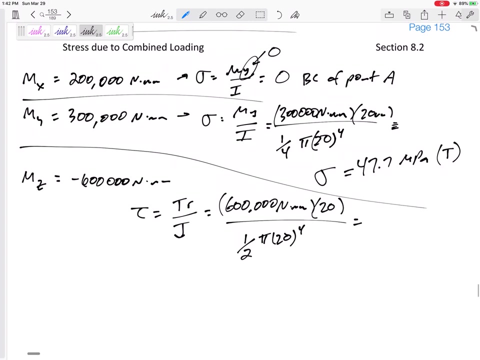 so at point a over j, the t is 600, 000 newton millimeters, the r, how far is my point away from the center of the middle dead middle center of rotation? uh, it would be the radius, and j is one half pi? r to the fourth. all right, one half pi? r to the fourth, so this would be a tau. 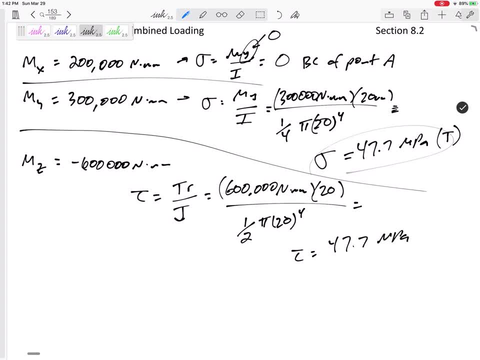 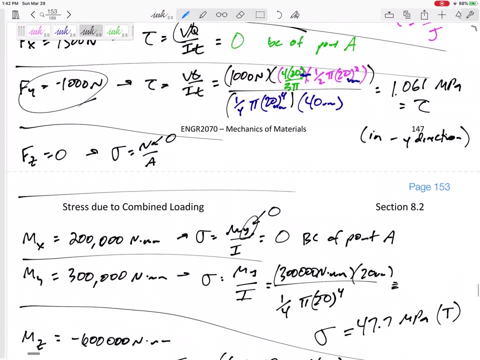 47.7 usually will not be the same value as what we got previously, um, but it was for that case, uh. so i've tau of 47.7. what direction, what direction? because you know i might could combine it with this one. i need to know the direction that it is in the direction. you see how i drew it right here. 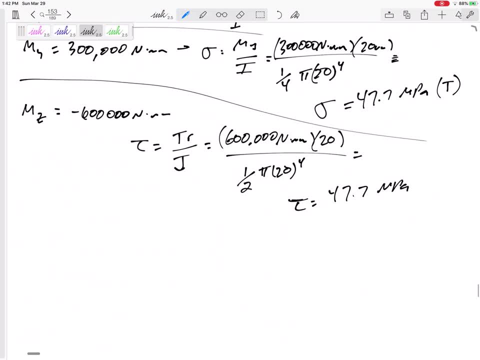 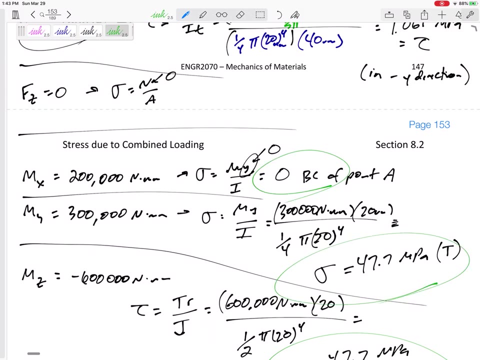 in the negative y direction. in the negative y direction, okay, we're not done, we, i mean we're we did. very good so far. right, that stress caused by that moment, that stress causes that moment: zero stress caused by that one. zero caused by that one, that stress and zero. so someone would be zero. 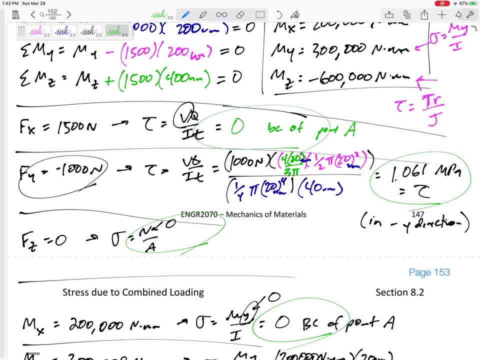 because it was zero to begin with. someone will be zero because of the point you're looking at now. you need to combine- that's the, that's the whole point of this section- combine all the similar stresses in similar directions. let me combine all the normal stresses together. 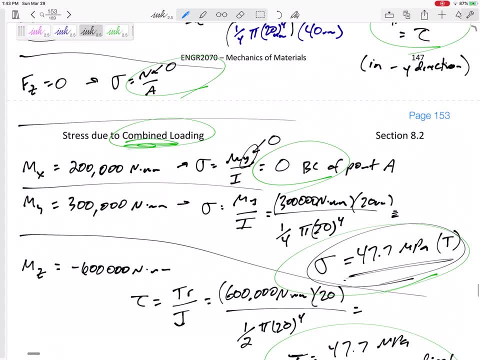 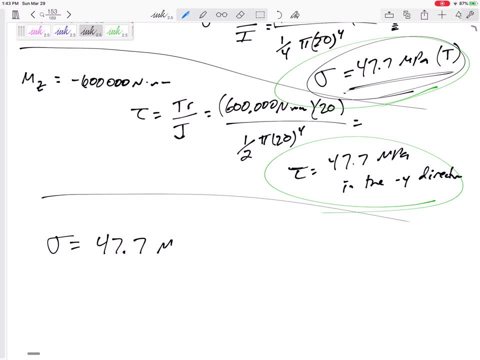 so this bending stress: 47.7 tension, okay, that one was zero, oh, and that one was zero. so all three of those, uh, there was actually only one. so 47.7 mpa in tension. that is my shear stress. at point a, at the cut aa, all right, but my. 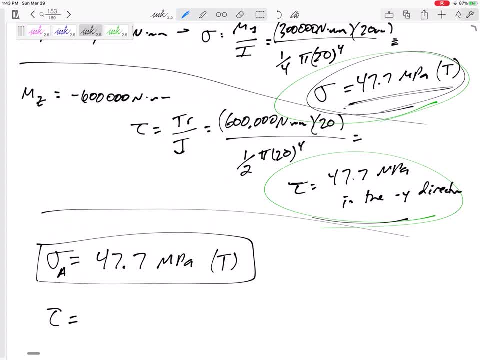 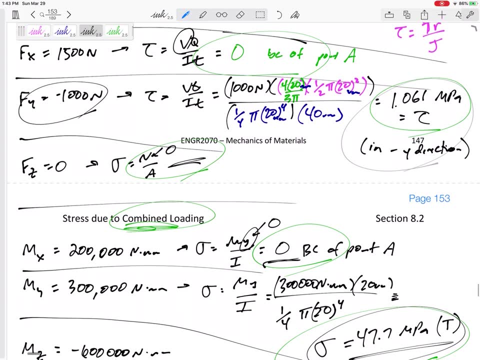 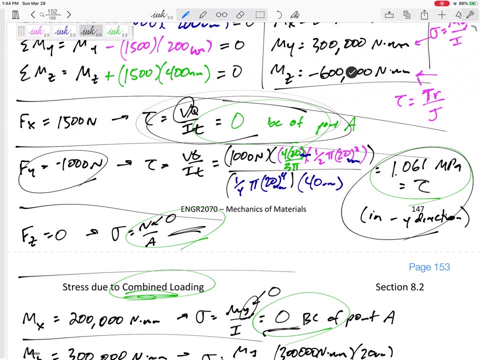 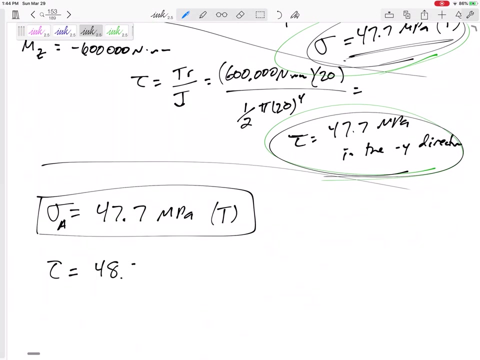 tau. let me combine taus. if they're similar stresses in similar directions, all right. so 47.7 in the negative y and 1.061 it all also in the negative y and then zero. that would have probably been in a different direction anyway, uh so, but anyway, i can combine those and i can. i can bind those that add up to 48.8 mpa. 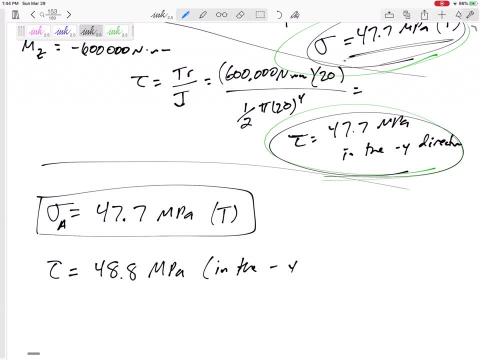 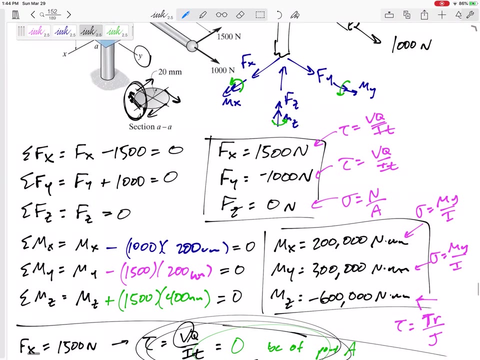 and i want you to put in the negative y direction, in the negative y direction, and that's it. that's it, we did it. but you know, take a step back. i'll let you do this on your own. go back, make sure you can find the internal forces. 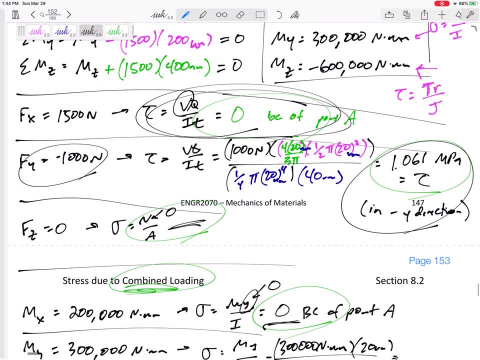 internal moments and then take each one of those and figure out what type of stress it is, uh, the equation for that stress. but then you got to think about what point you're looking at. sometimes it'll be zero just because you know that, that the shear stress at point a is zero for 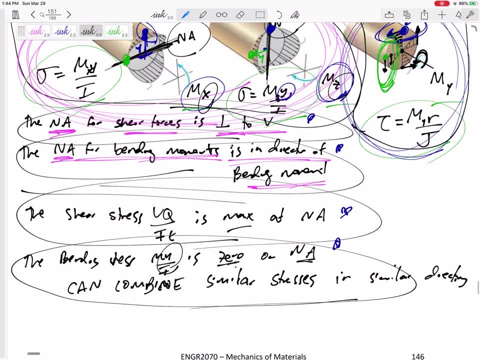 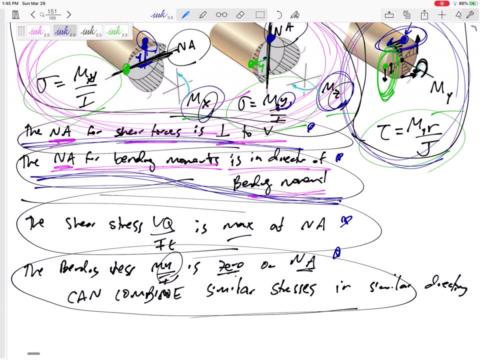 this one: um, go back and look at the, the, these, these, these two stresses, and i'm gonna show you these statements right here about where the neutral axis is for each of those and then what is happening at the neutral axis. That really helps me to draw the neutral axis in this scenario. 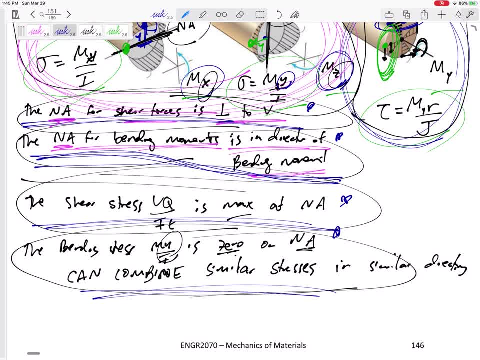 and then I'm like: oh okay, there's no bending stress happening at the neutral axis, So if I'm on the neutral axis then you don't have to worry about that. Or look at the neutral axis for my shear- and there is definitely shear stress on the neutral axis. In fact that's where the maximum 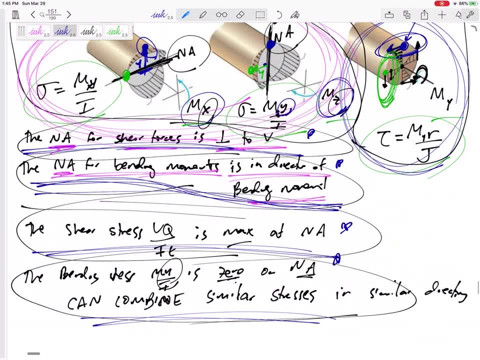 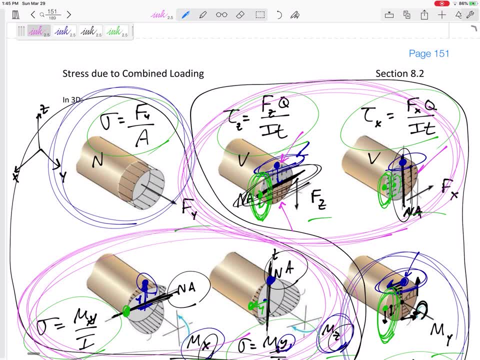 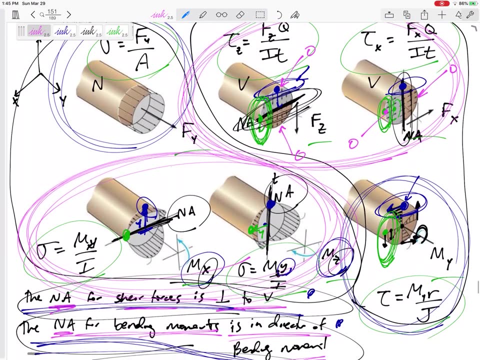 is going to be. But on those very, very leading and trailing, let's see, right here, yeah, on this leading and trailing edge, or in this case, right there and right there, those are going to be your zero points of shear stress. So, drawing those neutral axes and kind of figuring out what's,